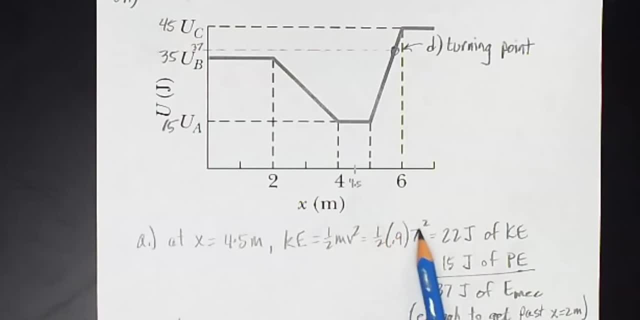 meters per second so we can figure out how much kinetic energy it has. Its mass is also given as 0.9, so I know it has 22 joules of kinetic energy And according to the graph, at this position it has 15 joules. 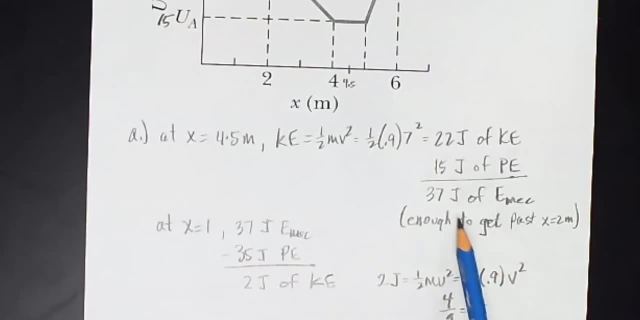 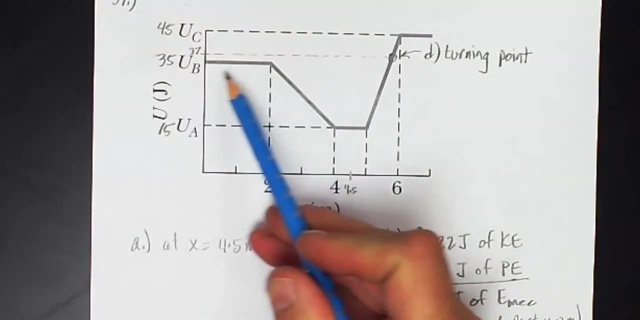 of potential energy. So that is a total mechanical energy of 37 joules. And if I were moving to the left I need to have more than 35 joules of mechanical energy to get past this point. So I will get past- x equals two meters and I'll have two joules of kinetic energy left over. 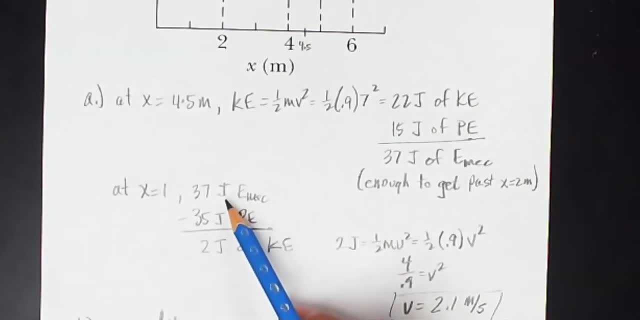 The difference between the potential energy at x equals two and the amount of mechanical energy that the particle has. So 35 of it is pe, two of it is ke. So two then is equal to one half mv squared. Solving that for v. 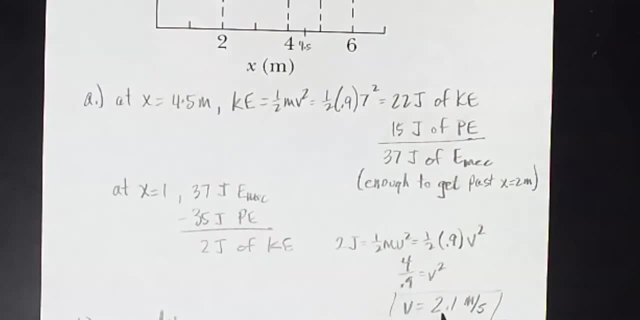 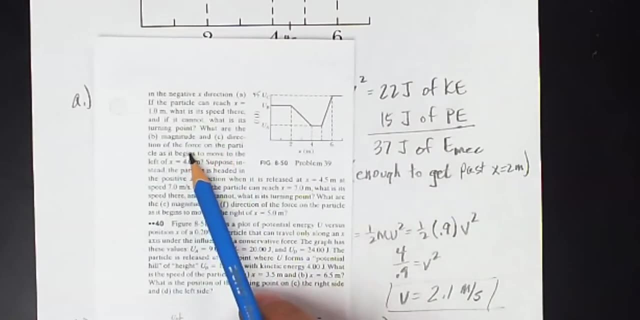 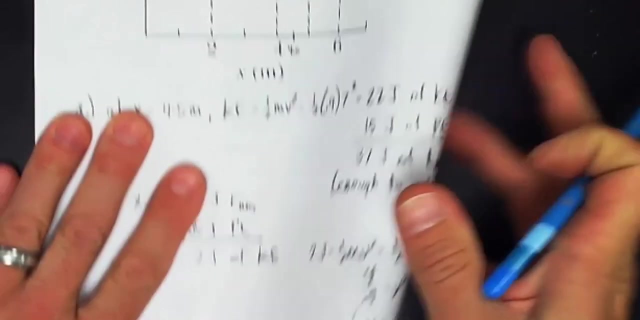 I see the particle is moving at 2.1 meters per second. Okay, parts b and c. What are the magnitude and direction of the force on the particle as it begins to move to the left of x equals four. So, as it moves to the left, it's going to move to the left of x equals four. 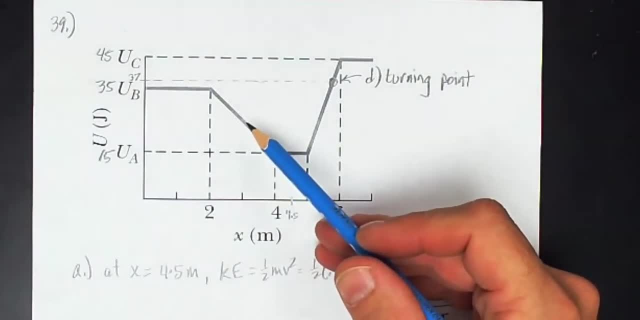 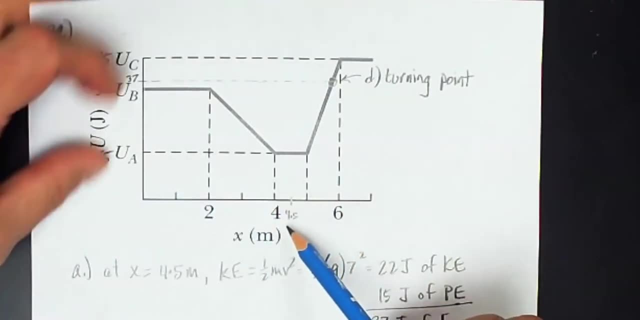 Perfect. If the energy we account to at this point in this region, what are the force and direction acting on the particle? Well, we remind ourselves that when we look at potential energy as a function of position, here's our equation that tells us it is the negative of the slope. 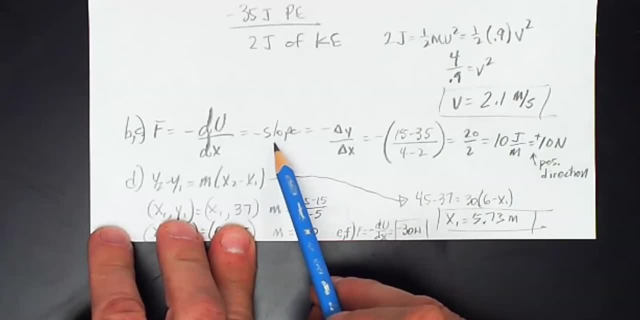 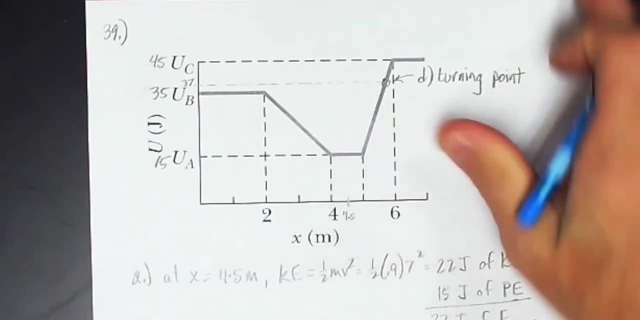 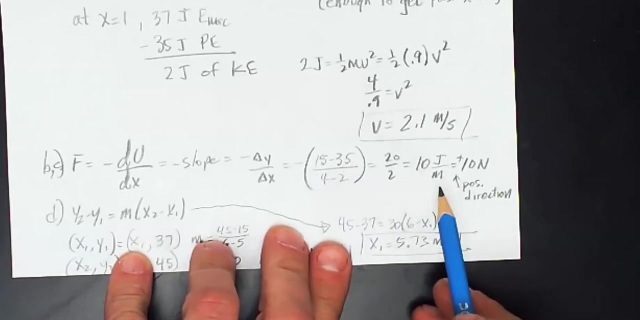 So, whatever the slope is, is the. The magnitude of the force and the direction is opposite of the sign of the slope. So in this region, we see, here we have a negative slope. OK, Perfect, Perfect, Perfect. OK, the negative of the negative, we get a positive. So the force is 10 newtons and it is in the 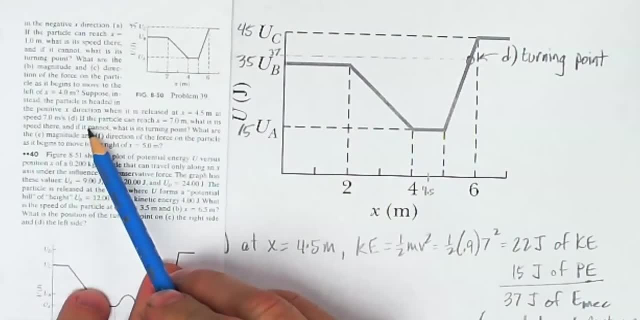 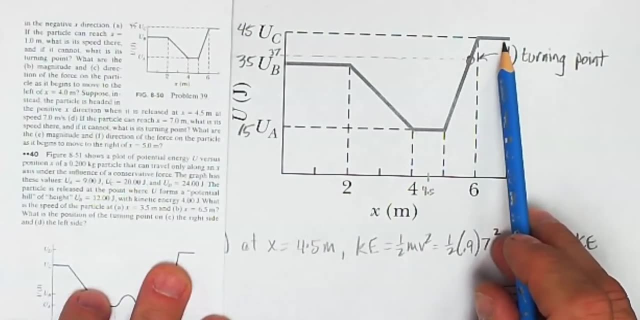 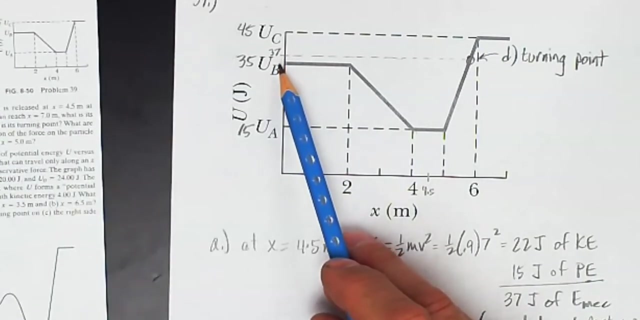 positive direction. Part D: if the particle can reach x equals 7,. what is its speed there? And if it cannot, what is its turning point? Well, I've drawn on the graph here. the total amount of mechanical energy we have in the system is 37 joules, and so this is as far as it can make it.